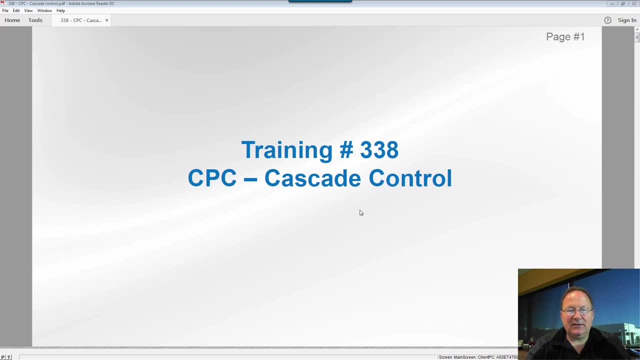 Hello again. this is Dave and I'm going to be training on CPC cascade control today, So you can follow along with the video. After the video, you might want to go back to the presentation and go through the finer details that are discussed in the presentation. I'm 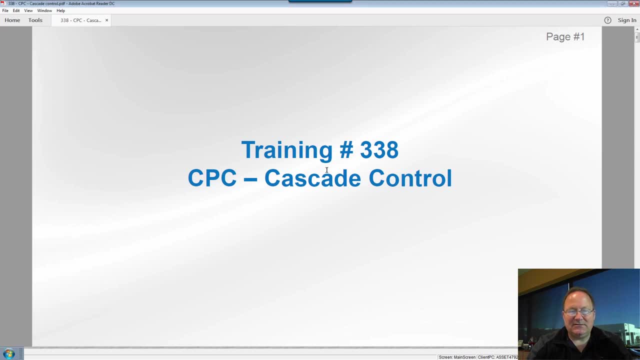 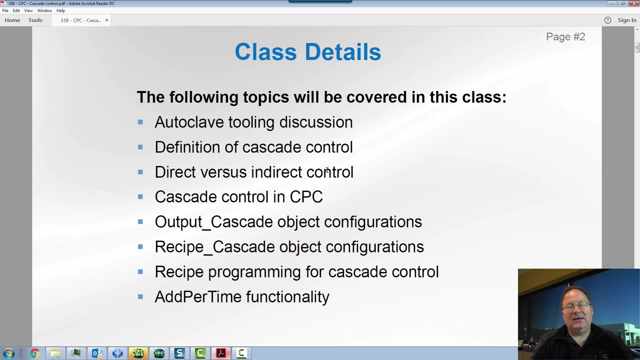 going to be brushing on most of these slides. So what are we going to talk about? We're going to talk a little bit about heating, how that occurs in the autoclave, and then we're going to get into cascade control, which is talking about direct, indirect control. 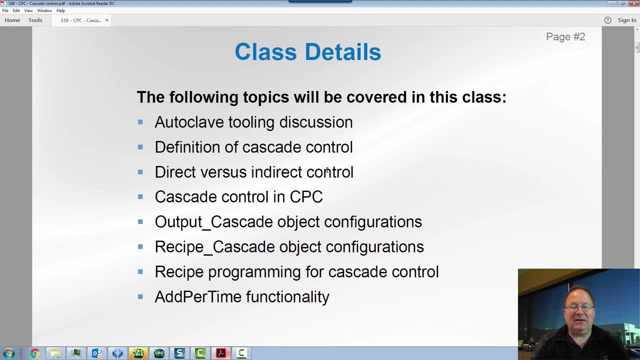 how cascade control is used within CPC, and then we'll be touching on the output cascade object, the recipe cascade object, and then we'll talk about recipe programming And then, at the very end, we'll also talk about an added function called add per time, which is the 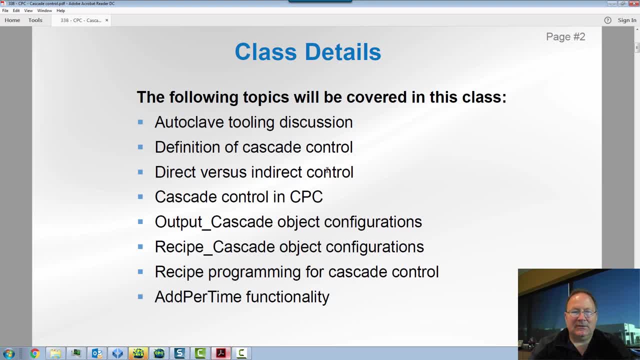 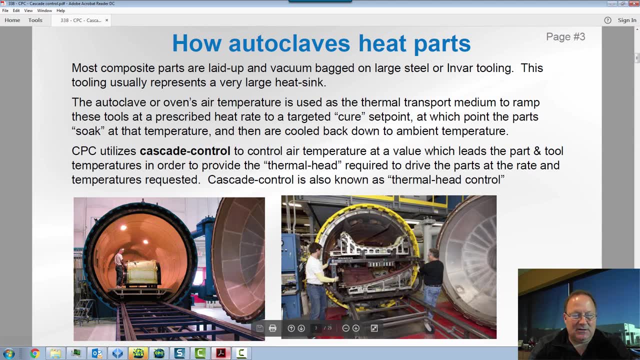 function used to provide an integral action to the cascades. So how autoclaves heat parts Basically. as you can see here, parts in autoclaves can be quite large and they're typically made of VINVAR or steel. They have a very large 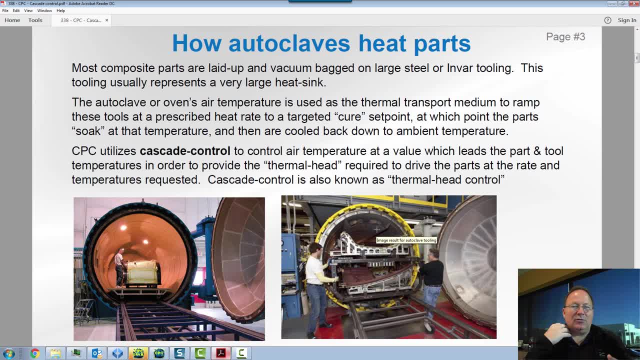 heat sink. So what we're doing in an autoclave control system is we're heating the air temperature and the air temperature is then transferring energy into the part, And so typically we're going to want to leave the autoclave in the autoclave control system and then we're going. 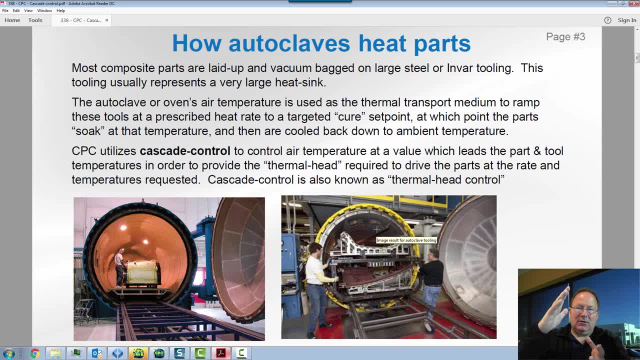 to feed the part with the air temperature. That is, the air temperature is going to ramp faster and at a higher temperature than the part temperature in order to drive the part up to the soak temperature or the cure temperature, And we use cascade control for that And that's. 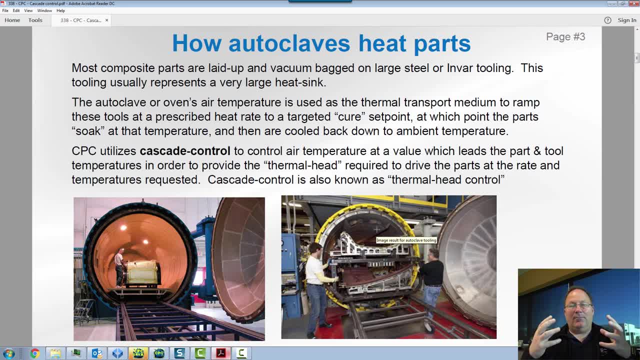 basically a method of controlling air temperature based on a part temperature feedback, And that's also called thermal head control. There's a lot of thermal head control in Europe. You're going to hear thermal head control in the United States. When we're talking about CPC, we're typically talking about cascade control. 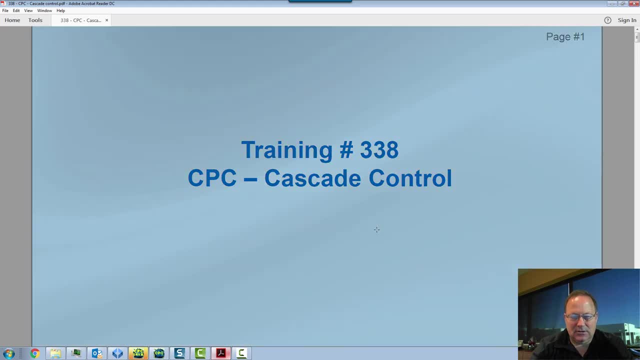 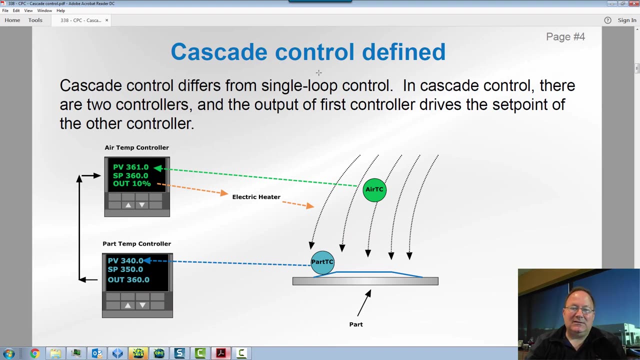 So let's talk a little bit about what cascade control means. Cascade control differs from the typical single loop control. Cascade control really is. there are two controllers. One is controlling the air temperature, The other one is controlling the air temperature. The second is controlling the part temperature and its output is really routed as a 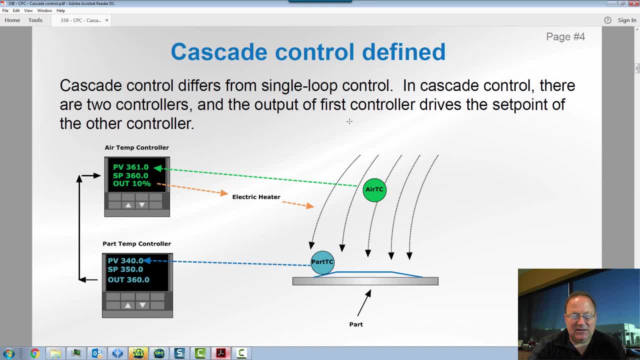 set point back into the air temperature controller. So you can see here that the part thermocouple, here on the part… here is your representation of the part- comes into this controller as a process variable. This has a set point, in this case 350 degrees, And its output. 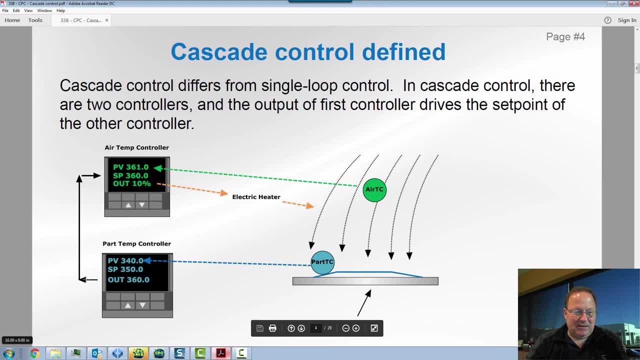 is not a percent output, but it's an actual temperature, which then gets routed over to the set point of the air temperature controllerischen. goodbye, resuscitation, schw runt. er hat strictly at which point, that is, controlling air TC at a higher value. 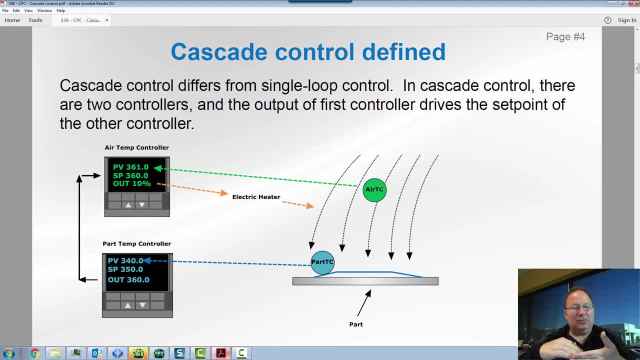 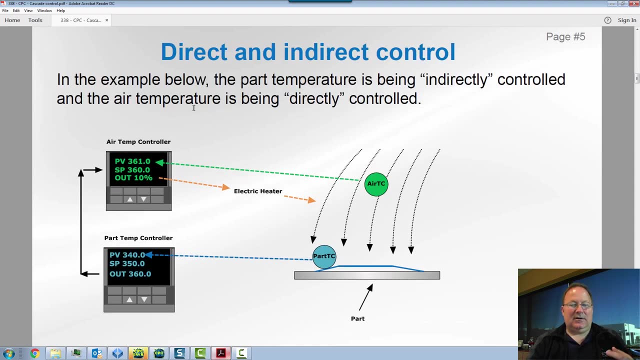 So, basically, if we want the part temperature to be at a certain value, then we're going to put air temperature either above or below, depending on if we're heating or cooling. Now this is also referred to as indirect and direct control. 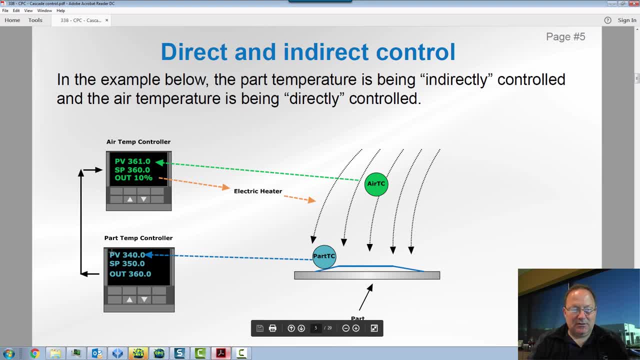 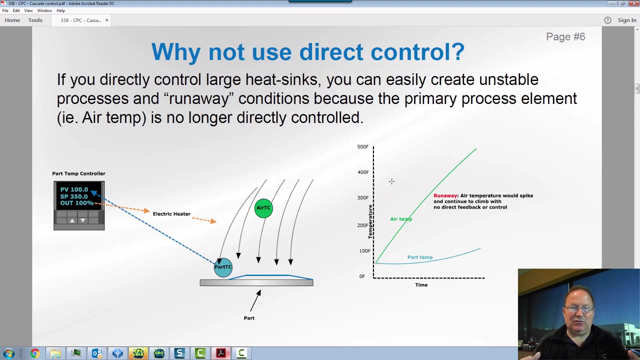 So we're indirectly controlling part temperature indirectly by directly controlling air TC. So part control within CPC is always going to be an indirect control method And we're not typically looking at the part thermocouple and driving a heater signal. If you do direct control of a part you can end up with some problems. 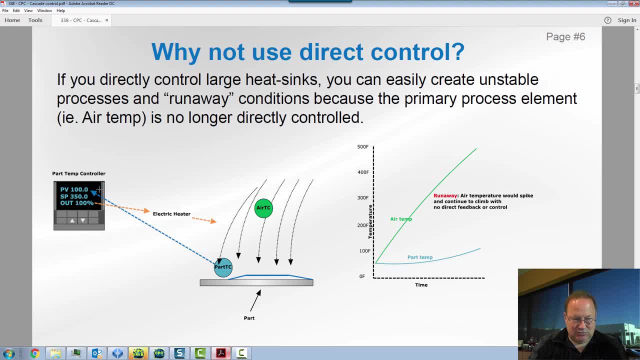 This diagram shows Part thermocouple coming into a controller, And in this case the part is at 100 degrees, The set point is at 350.. So we're going to end up, obviously, with a 100% heating signal. 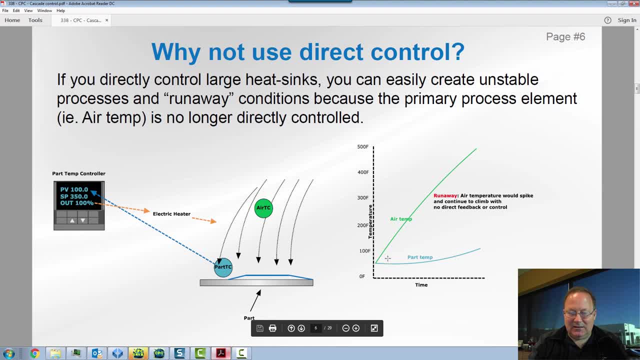 And what will happen is, even though the part temperature begins to heat, the air temperature will just keep moving up, up, up, up up at 100% heating, And that's considered a runaway Because basically there would be no direct control of air temperature. 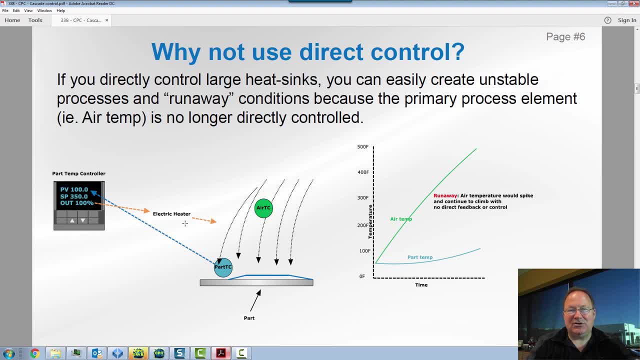 It would just be linked Basically To the operation of the heater, And so this is why direct control of large heat sinks is usually not a good idea, Because you end up with a runaway condition of the air temperature, And another reason why we use cascade control. 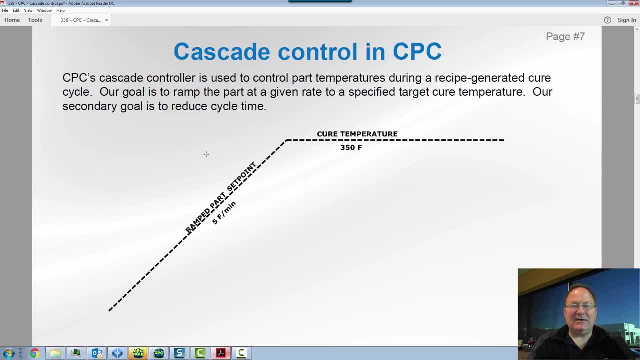 Okay, So cascade control in CPC. Most of our applications are going to be ramping a set point at a given rate. Most customers have a specific rate requirement. It might be 2 to 7 degrees of methane Or 1 to 5 degrees a minute. 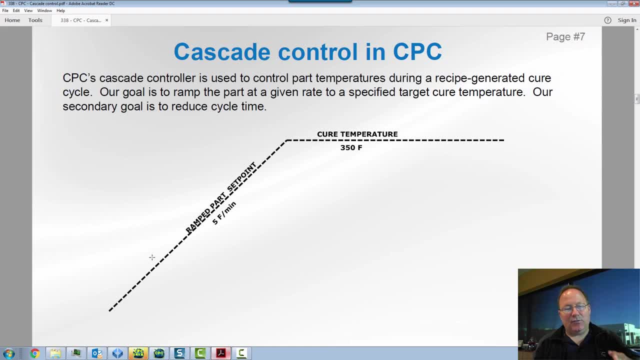 So there will be a lower tolerance and an upper tolerance of the rate, And then we'll go up to a specific temperature And there might be a single temperature or it might be multiple temperatures where you're basically ramping twice And in some cases they might ramp three times. 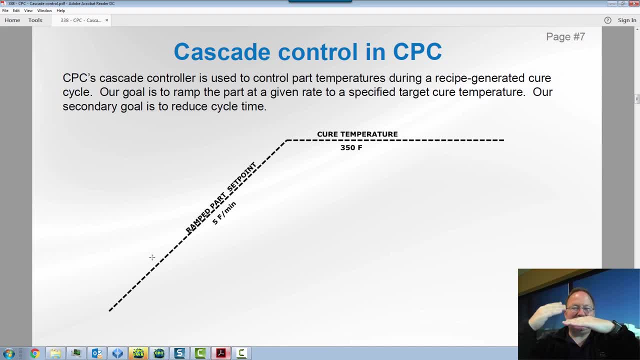 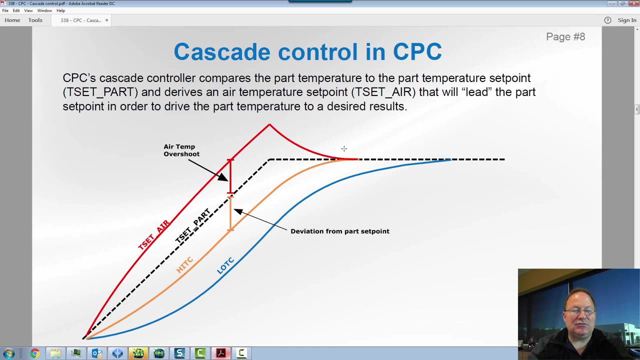 The final temperature typically has a plus minus tolerance. So in this case I'm showing a 350 degree. Normally you're going to see a plus or minus 10 degree tolerance on that. Okay, On that type of control, And what we do in a typical cascade control is the CPC cascade controller will compare the part temperature set point. 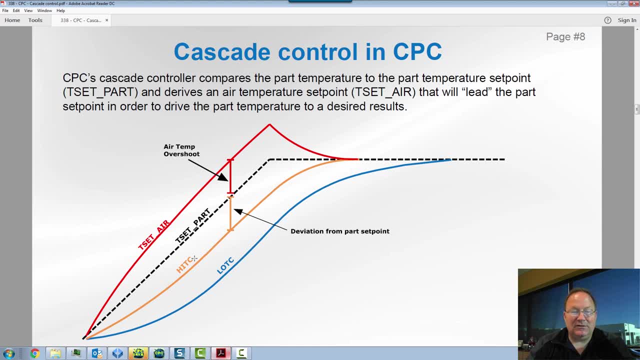 With the actual part thermocouple being controlled, In this case high TC, And based on that it will adjust an air temperature set point above the part temperature set point And you can see that this, This value, here we consider air temperature overshoot. 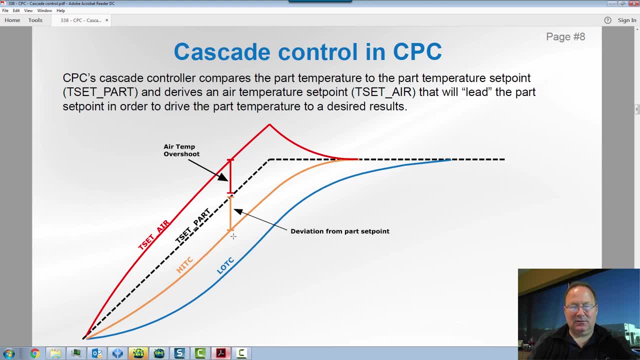 And this value here is deviation from part set point, And so for the rest of the training we're going to be talking about overshoots and deviations, So just remember that the deviation is the part set point minus the control thermocouple value. 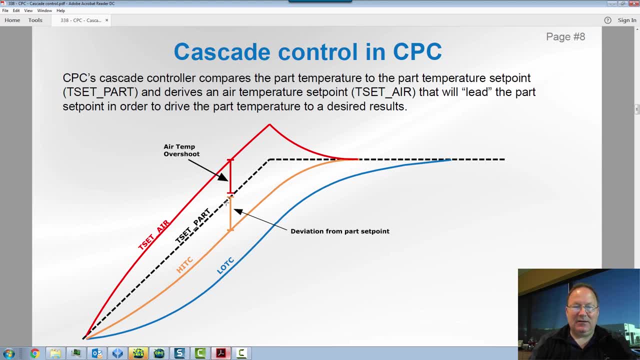 And the air temperature overshoot is always going to be on top of the part set point. Okay, And what you see here is We're driving that part temperature And as the part temperature comes up to final set point, the air temperature will come down, converging at set point. 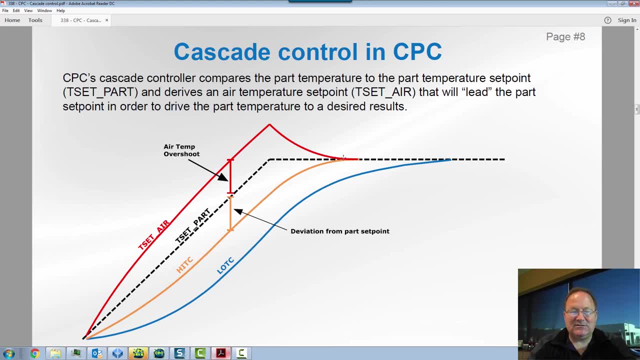 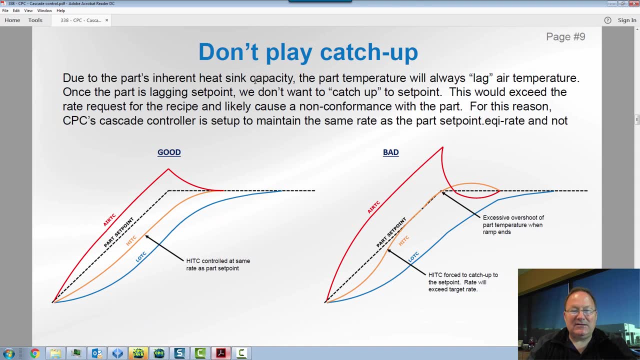 And that's a typical cascade shape that we're going to see in a trend. Now, obviously, due to the part's inherent heat sink capacity, the part temperature will always lag air temperature Once that part is lagging set point. we don't want it to catch up to set points. 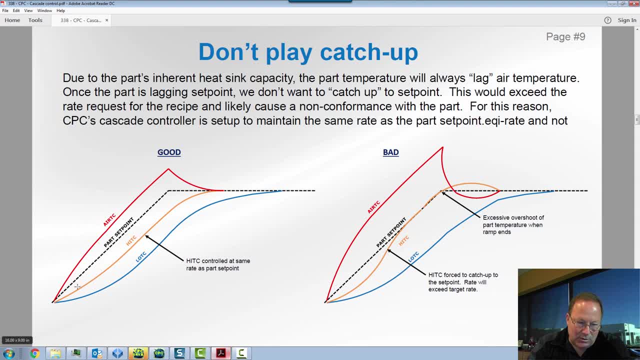 So what you see here, Even though part set point is here, We don't actually want this to increase and catch up, like you see here. Okay, Because what will happen here is, even though I'm back on the set point line with my part, thermocouple. 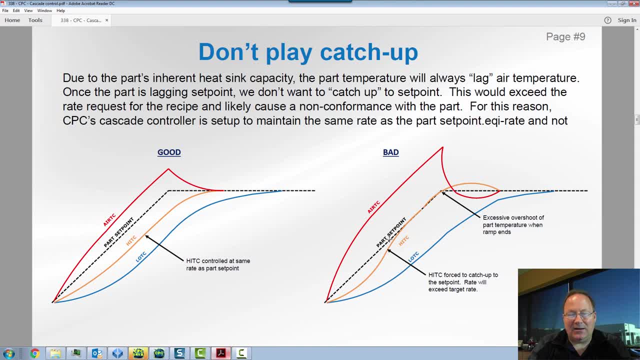 In actuality, I'm exceeding my desired rate by a lot, Right, Because I've asked for, in this case, 5 degrees a minute, But in order to catch up, it's going to go 6,, 7,, 8 degrees a minute. 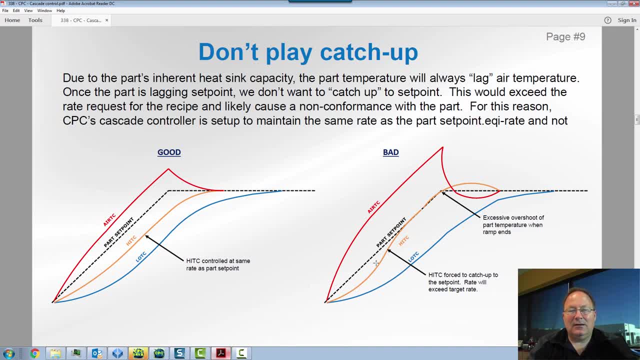 And so we're actually doing that. We're deviating from the plan. So we are not necessarily expecting this line to be on top of this line during a ramping segment, Because of the fact that we would have to exceed rate, And so our cascades are always designed to put that ITC at the same rate. 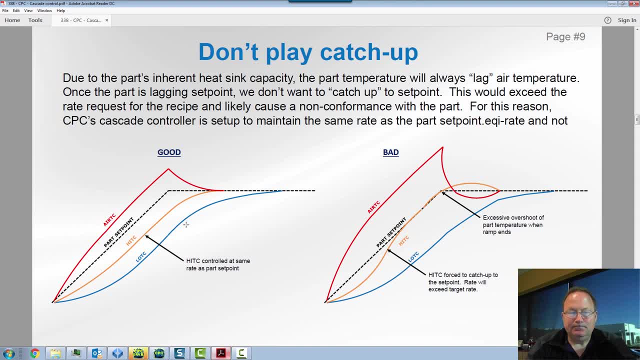 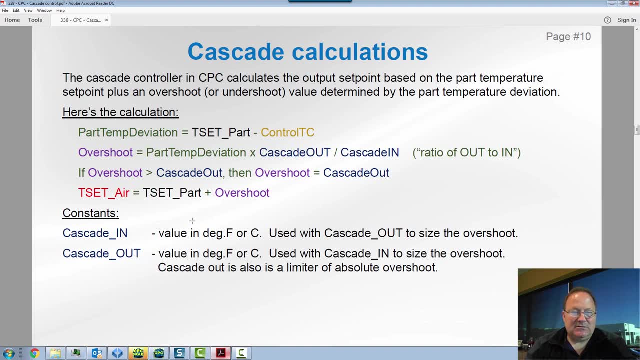 But not necessarily catch back up on the line. Okay, So here's a cascade calculation. Basically, what we do is we determine a part temperature deviation And that's going to be the T set part, Which is the part set point minus the control TC. 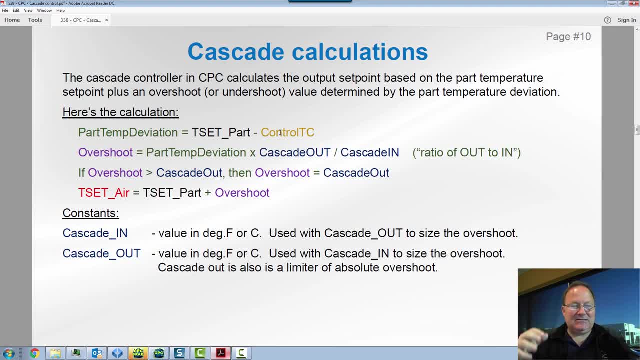 Which would be whatever is being selected. So if it's the high TC, then it's going to be the highest of the part TCs, And so basically that is going to be the deviation, And the overshoot then is that deviation multiplied by the ratio of cascade out to cascade in. 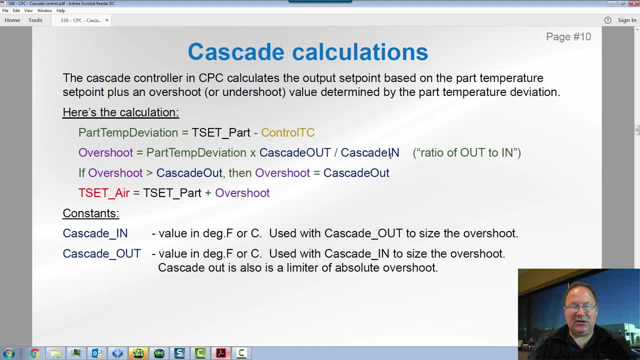 Okay, And basically that out to in ratio. These are two constants That are called cascade in and cascade out. They're both in degrees units- Degrees F or degrees C, depending on the system- And in addition to the actual ratio, Meaning that the overshoot is going to be a ratio of those two constants. 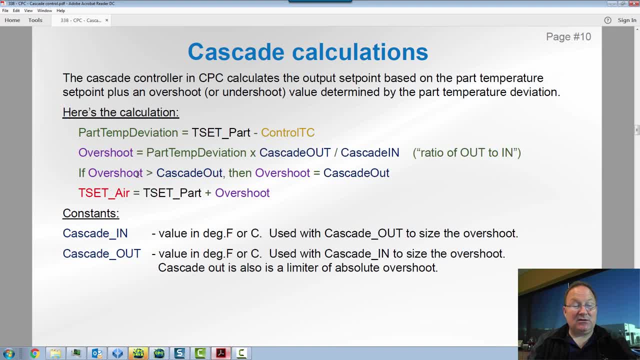 One of the constants. cascade out is actually a limiter as well. So if the overshoot exceeds that cascade out value, It will then equal that cascade out value And basically T set air then becomes the part temperature deviation Plus that overshoot. 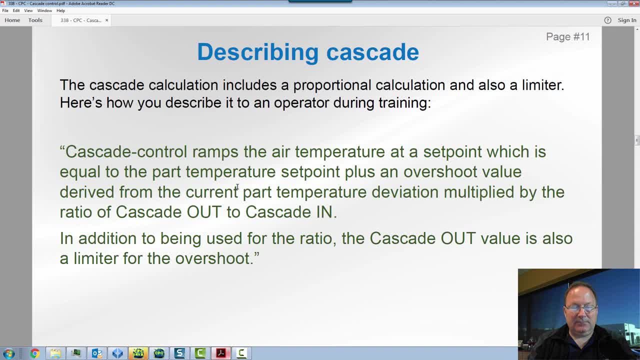 Okay, So how does that look in? So basically, when you're talking to an operator, You would want to say: okay, cascade control ramps the air temperature At a set point which is equal to the part temperature set point, Plus an overshoot value derived from the current part temperatures deviation. 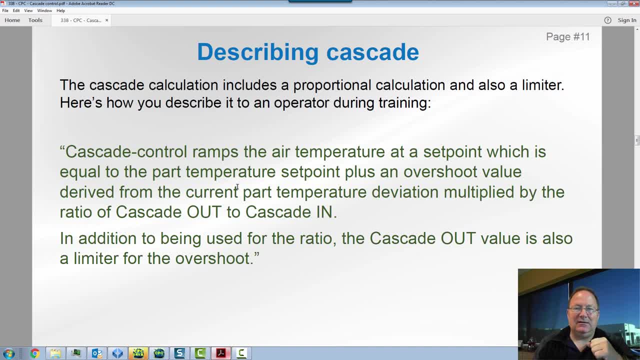 Multiplied by the ratio of cascade out to cascade in. And then you would remind them that that cascade out parameter Is also the limiter of that overshoot. Okay, So really it's all about the ratios. So you know a one to one ratio. 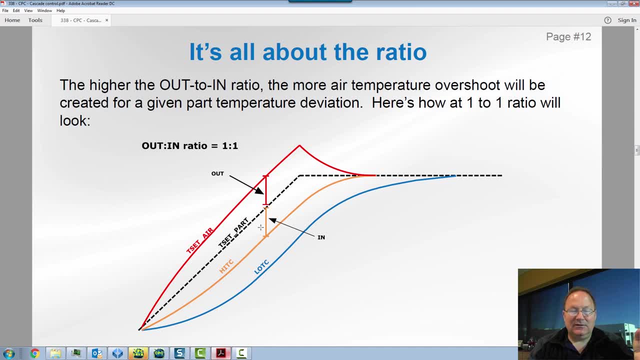 We would expect for every one degree deviation, We would end up with a one degree overshoot, And so this is typically what you're going to see with a one to one ratio. A one to one ratio is a fairly conservative ratio on control. 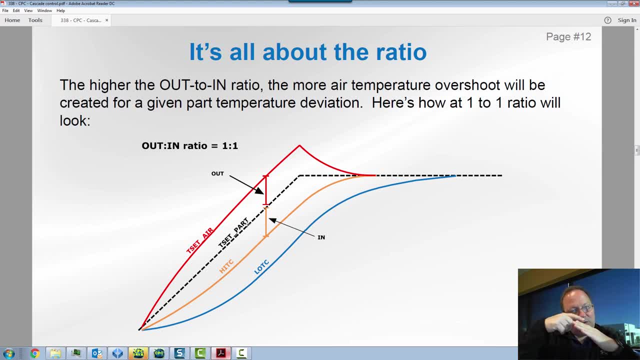 Because even if a thermocouple is moving a little bit with noise, You're not going to see big changes with air temperature, But you are going to end up with A lot of thermal head Right, Which is basically This additional momentum being used to drive that part thermocouple. 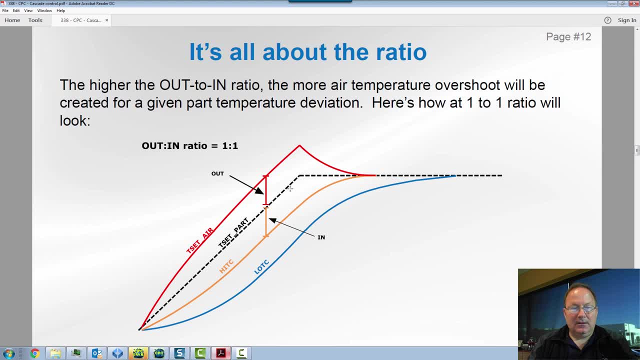 Up to set point Now, As you increase your ratio of out to in. Okay, And again we talked here Cascade: out is this overshoot. It represents the out version Or the overshoot part, And in is the. Is the? 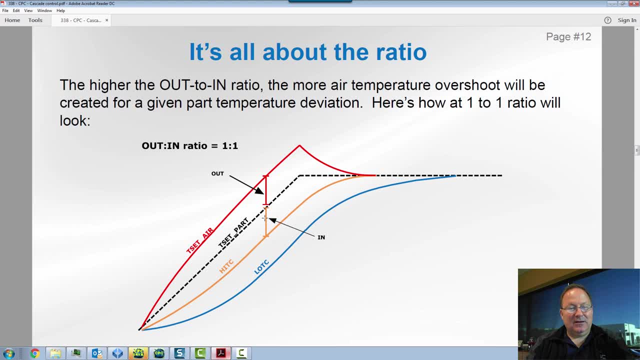 Is the deviation part. As we increase the out to in ratio, Cascade out becomes larger than cascade in. We're going to see More air temperature overshoot for a given part, temperature undershoot. Okay, And so here We end up with a deviation. 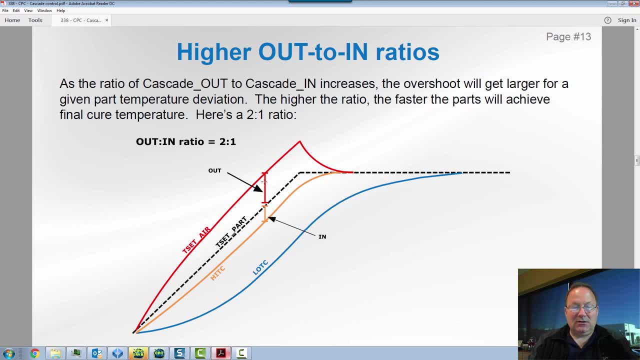 A smaller deviation Results in a larger overshoot. Okay, And that's a two to one. Now That That is going to heat your part up faster, It's going to shorten your, Your cycle time, Which is all good. 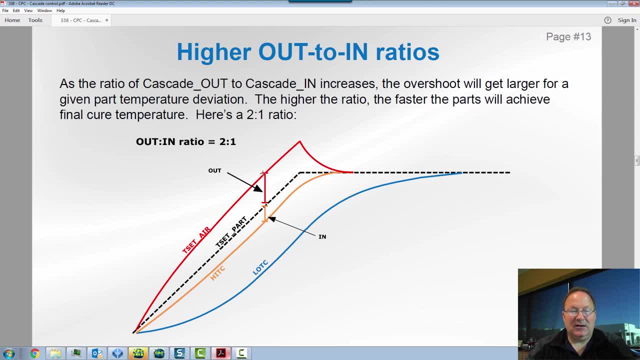 But You're going to end up with a one to one ratio. Okay, And that's a two to one, Now That That is going to heat your part up faster, It's going to shorten your, Your cycle time, Which is all good. 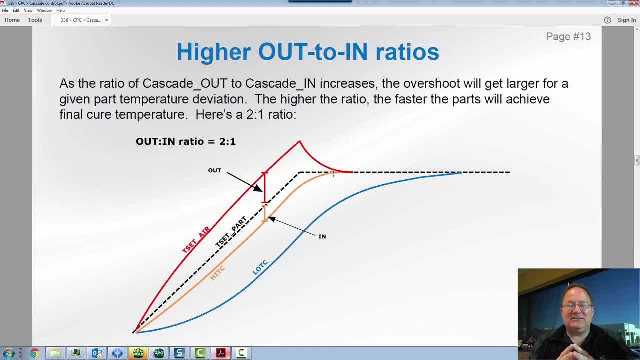 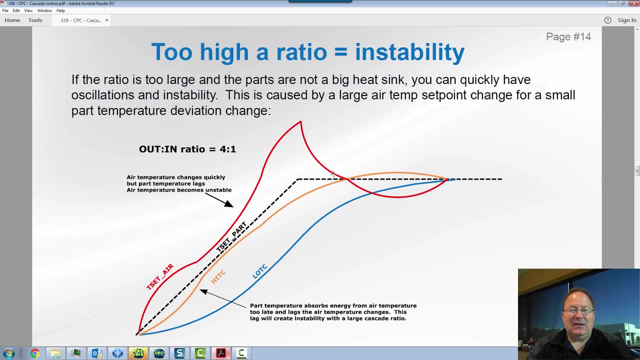 But What you don't want to have is A situation where you say, Oh, If two to one works, great, Let's try four to one Or six to one, Because What will typically happen there is Instability The higher the ratio. 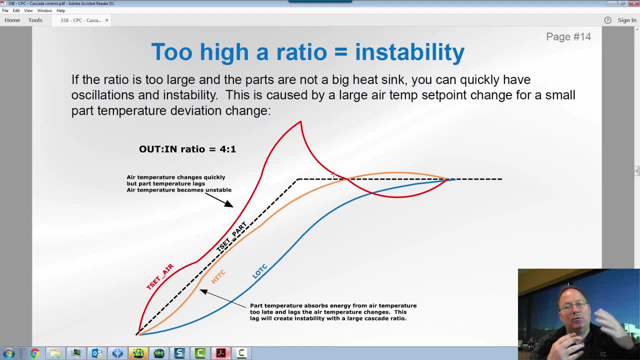 You're going to become more and more Unstable. And what? What occurs there is Basically, For every small change in a thermocouple, In a part thermocouple, You're going to end up with a large change In air temperature. 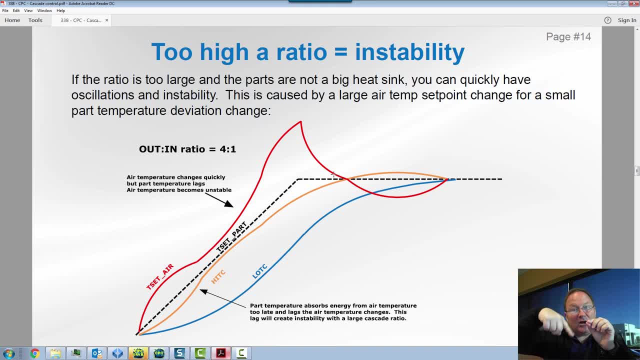 And You, You can end up with Some very, Very Shorten your, Your cycle time, Which is all good, But Very Odd looking trends Because, Because As that, As that part thermocouple Starts to 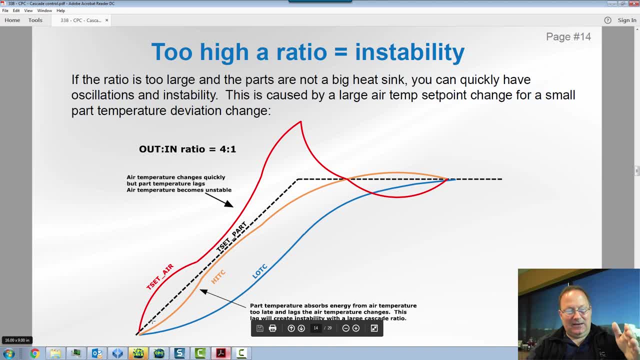 Deviate From set point, Air temperature is Going to rocket up And then Part Temperature is going to react At some point And come up, And then Air temperature is going to Come diving down And you're going to end up with 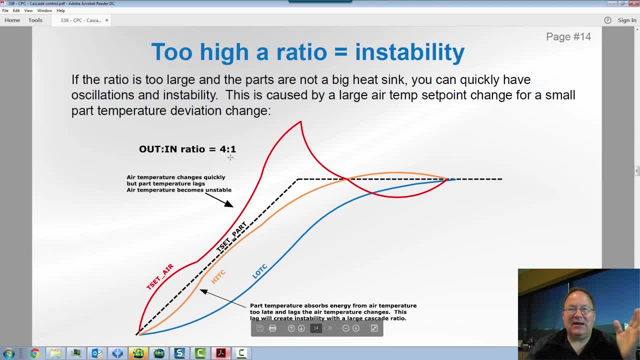 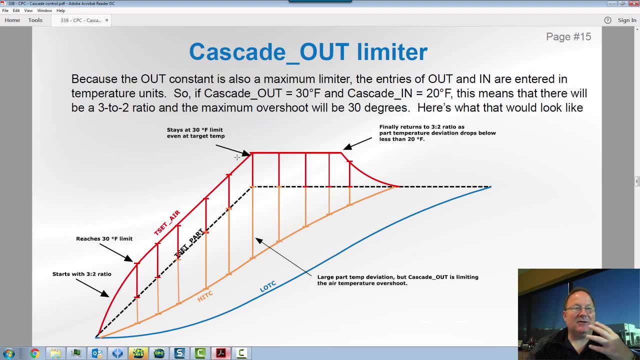 A very unstable condition. Okay, So It. Usually You're going to want to be Very careful about About setting out In ratios. So I I talked about the fact That the Cascade out Constant Is. 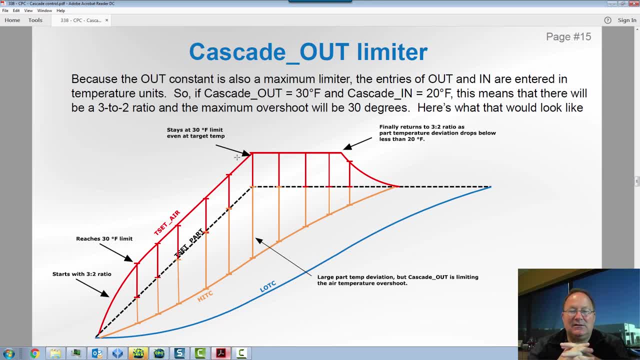 A limiter As well As a ratio Creator, And so, Because it is Is a limiter, You can You can use it To Provide A little bit of a A check On how much air temperature. 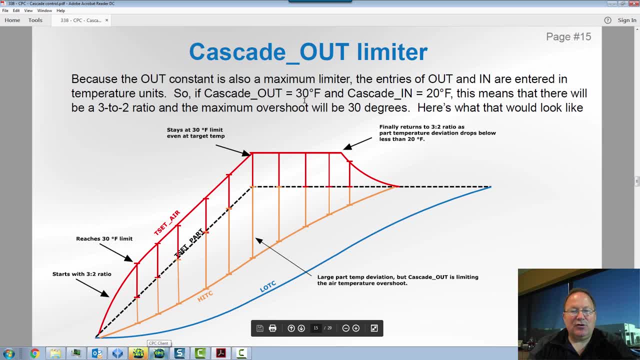 Actually goes into your Process And you can see here That That We We are setting A Cascade out As my output Cascade out value, Which will limit The maximum Overshoot To thirty degrees, And so 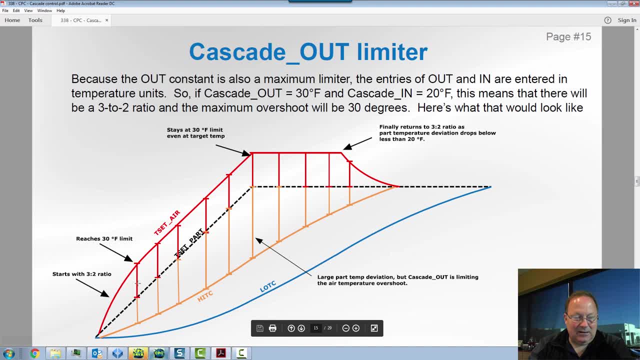 Although At my part Begins to deviate. And I can. I can Slow, You know Slowly- build my, My overshoot. At some point We're going to reach A thirty degree limit And it'll just. 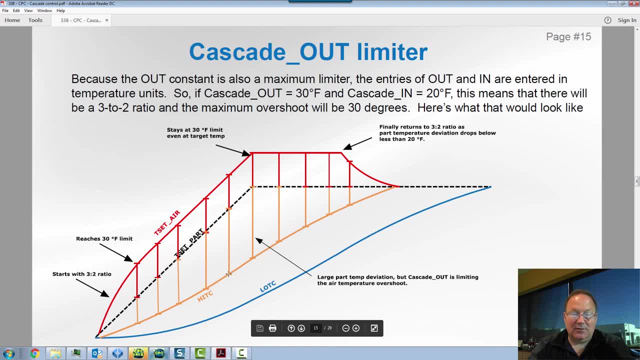 Maintain that, then For the For the rest of that ramp, Even though My, My actual thermocouple Has deviated far below What would be. And then, As we come up, You'll, You'll, You'll see that. 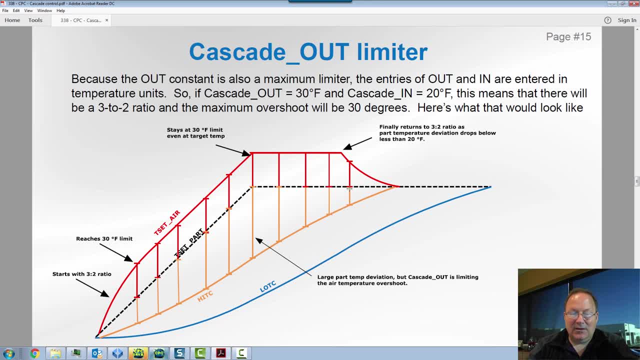 It'll clamp it At thirty degrees Above set point here. Then At some point When your part Does come Within the range Of a two to three ratio Within the thirty degrees, We're going to start Dropping back down. 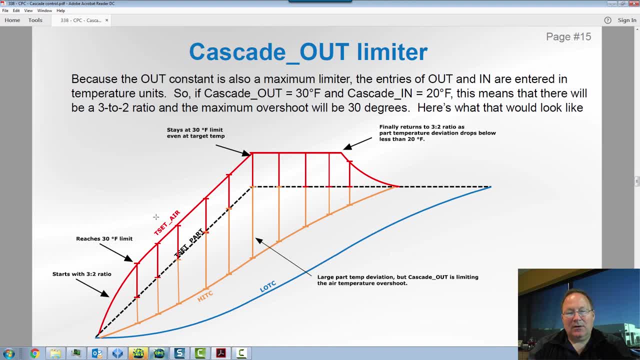 And so This is What you're going to see In a typical Cascade out Limited Process. Okay, Now Do Do people Use that? You can Use the Cascades For the Limits Other. 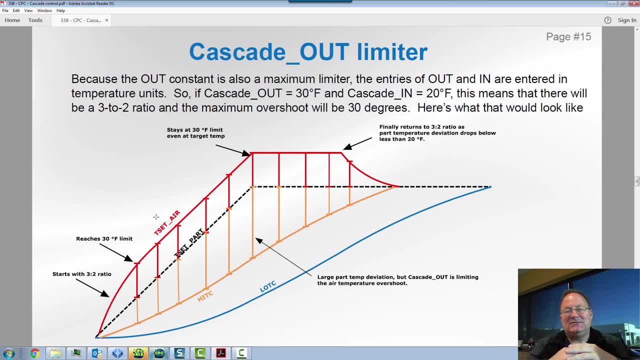 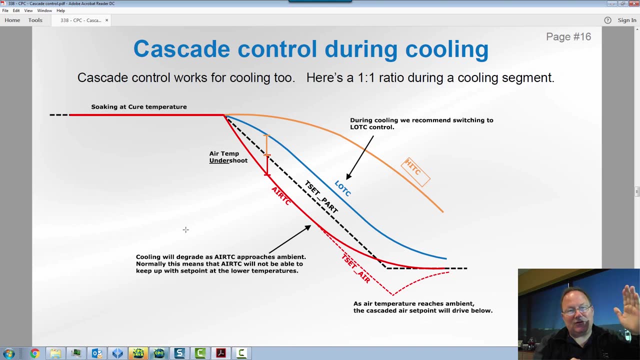 Customers Go ahead And set The Cascades Much Higher And then Allow The Air Temperature Limiter To To To Work. It's, It's Magic In the Recipe. 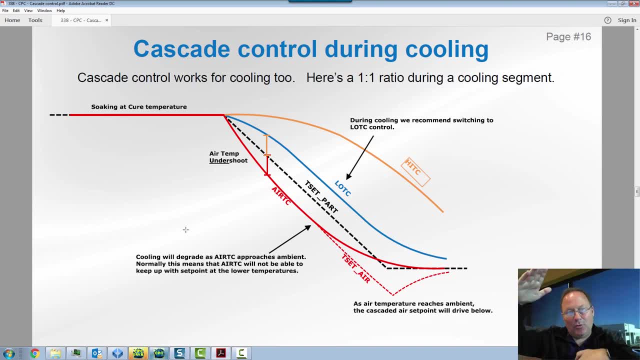 So Cascades Also. The Air Temperature Lower Than The Part Set Point In Order To Drive The Low TC At The At The Given Rate. 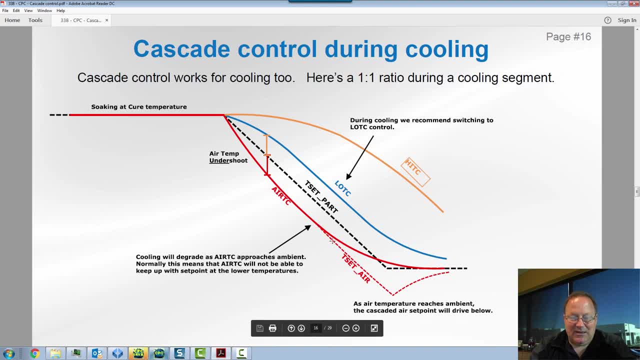 But Obviously, With The, With You Know The Set Point Down Here, We're Going To Be Limited For The Air TC And You're Typically Going 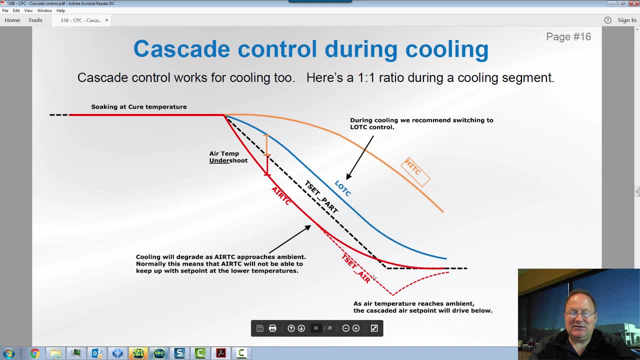 To See This, This Type Of Action, Where, Where We're Able, We're Only Using Ambient Temperature Water. So This Is What You're Going To. 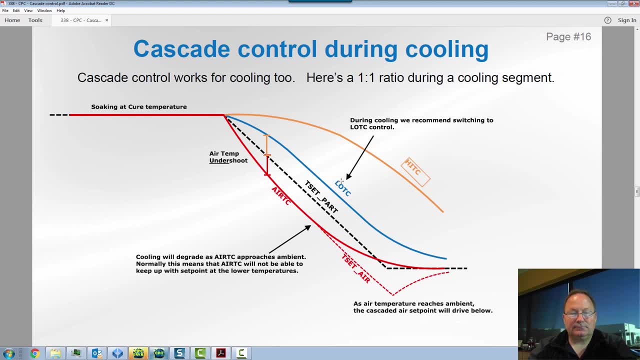 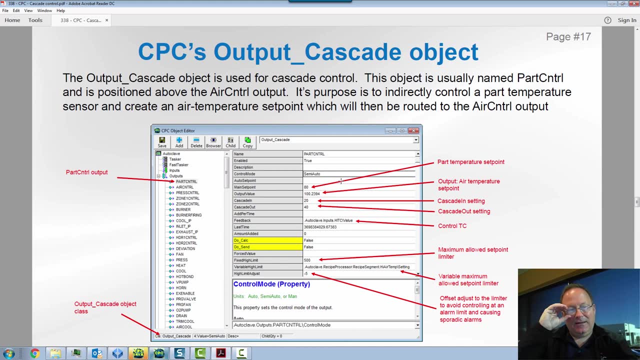 See Okay, And When. One Thing To Note Is: During Cooling, We Want To Control By And We Call It Part Control. It Can Be Called. 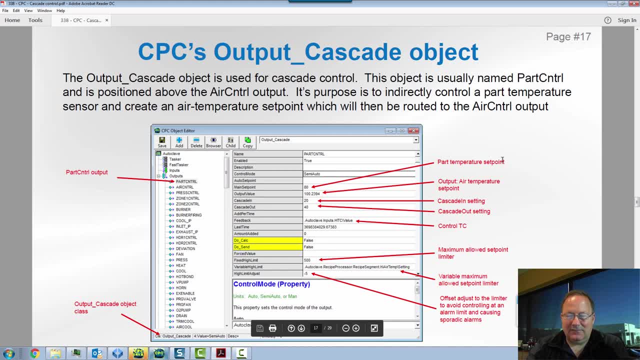 Other Things, But This Is Just The Standard. We're Going To Call It Part Control And We're Going To See What Happens When We're 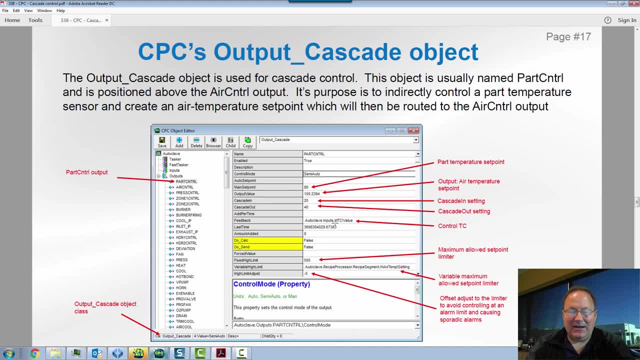 Calling It That, We're Calling It In The Out Of The Case And And You're Going To See What Is Happening And We're Going. 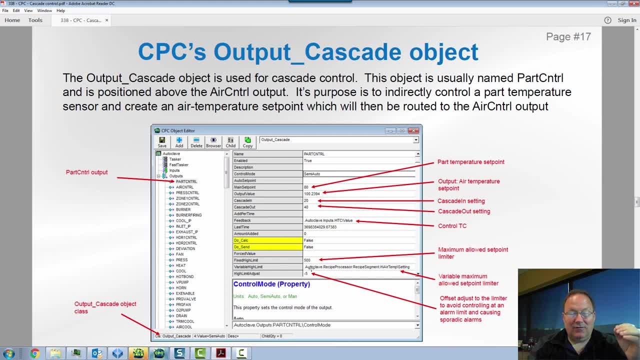 get higher than 500 degrees. and then we also have a variable high limit, which is usually tied to the recipes max air temperature setting with a specific adjustment for avoiding alarming. So that's the output cascade object. You're going to find this in virtually every configuration where we're controlling ovens. 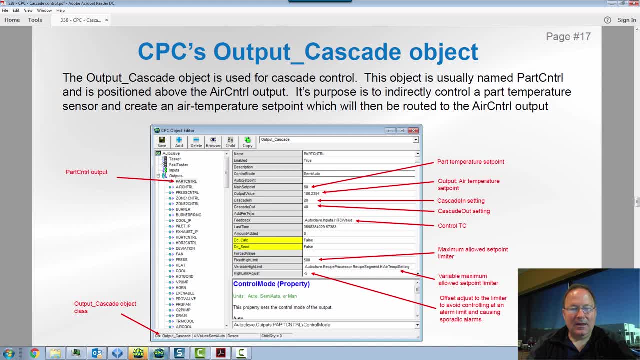 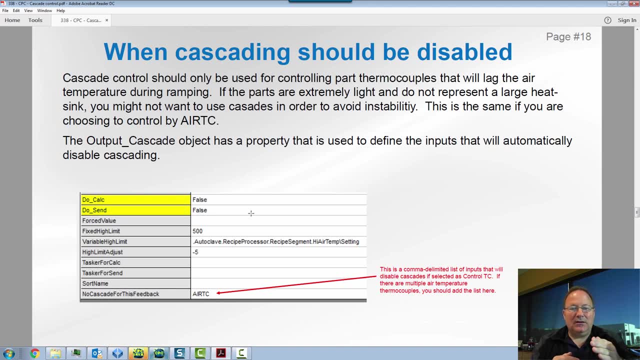 or autoclaves or that type of thing. When should cascades not be used? Well, there are cases where cascades again are used to drive part heat sinks and if a part is very thin, let's say you're running some very thin aluminum sheets. tiny little. 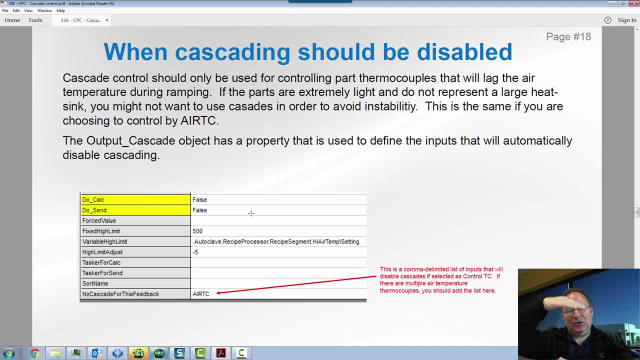 aluminum sheets. they're going to react to air temperature so quickly that you don't want air temperature to be sort of driven higher than the set point. So there are cases where you're going to want to choose to not use cascades. That can be selected in the recipe. but we also understand that if an operator selects 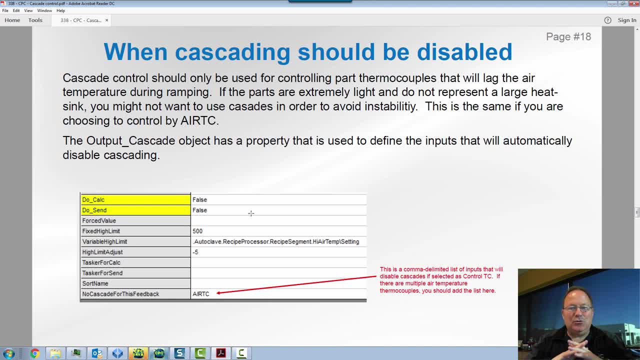 air TC as the controlling thermocouple in a recipe. we definitely do not want to cascade air TC because that will become the indirect controlled unit and then we're going to pass a set point up to the controlled unit, which will be air TC. So the system has to have a property that lets it know which inputs. it should not cascade. 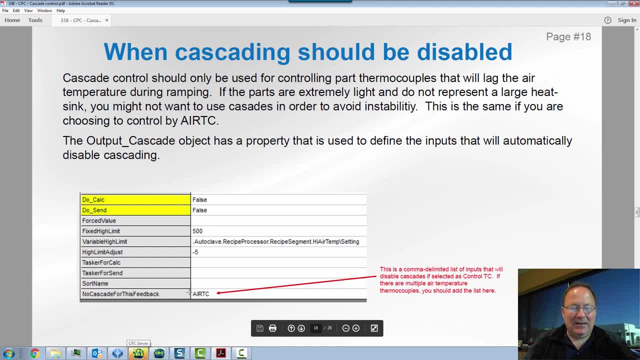 and so there is a property called no cascade for this feedback in that output cascade object, which is used to define a list of inputs that are not going to be cascaded, And so it's almost always going to be air TC, but if you have multiple air temperatures, 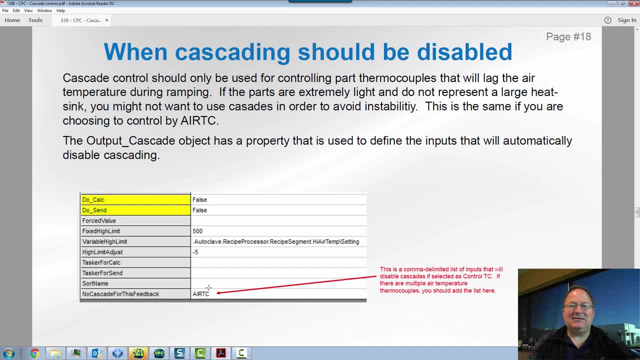 you might have air TC one, air TC two, air TC three. you want to put that as a comma delimited list. That way, if the operator happens to put air TC five or air TC three as a control thermocouple, the system won't attempt to try to cascade and control that. 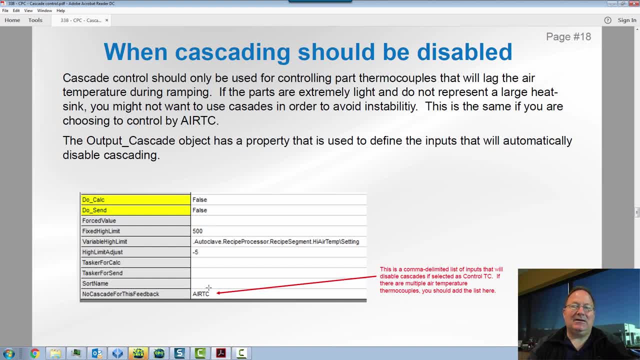 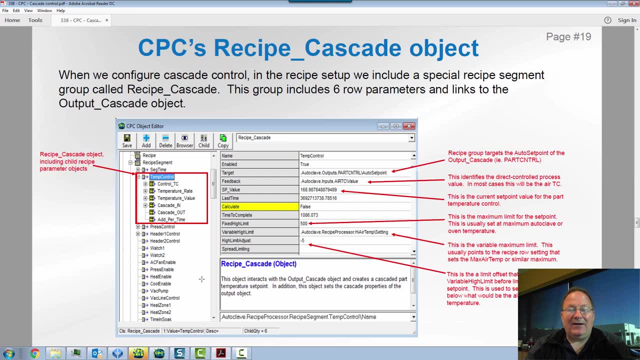 It will know that. okay, that's one of the list items that I should not cascade control. So we talk about recipes. Well, the recipe will now have to have a recipe cascade group in there, and so you can add a recipe control object. Okay, 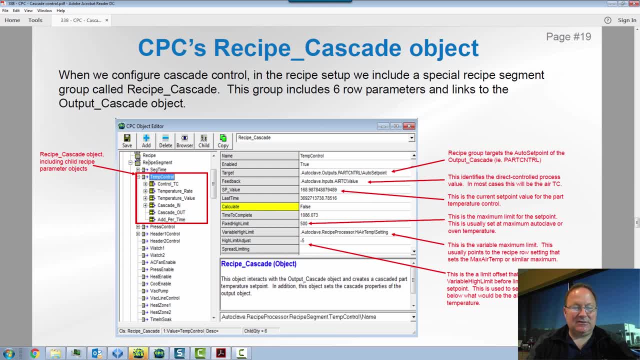 Or a recipe cascade object to the recipe segments object here And that will have six properties or six rows beneath it: Control, TC, temperature rate, temperature value, cascade in, cascade out and add per time. And that recipe object is going to be targeting the part control output that we talked about. 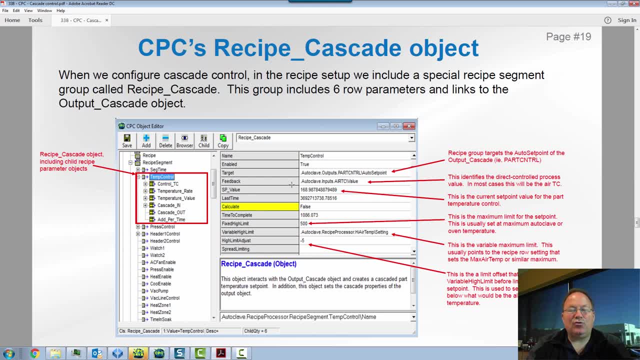 the auto set point of that. The feedback here is the primary feedback. So remember, We talked about indirect control and direct control. So this is the direct control feedback of this cascade control and in this case it would normally be air TC. Okay, 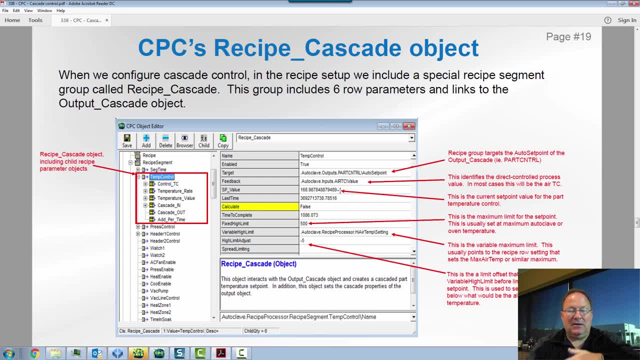 And the set point value. it will always display the set point being generated by that ramp, so controller here, which is the temperature rate and value. and then what this object does is, when it's running, it's going to transfer a lot of these properties over to the output. 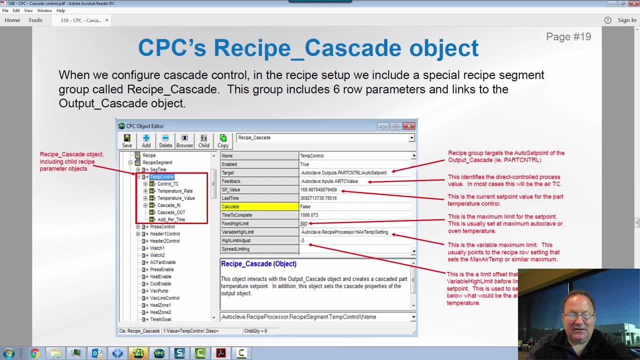 object: Okay, And we have again the same fixed high limit and the variable high limit that we talked about before. So this object again you're going to see it in primarily or most of all the configurations that you deal with. it will have a temperature control cascade object in the recipe. 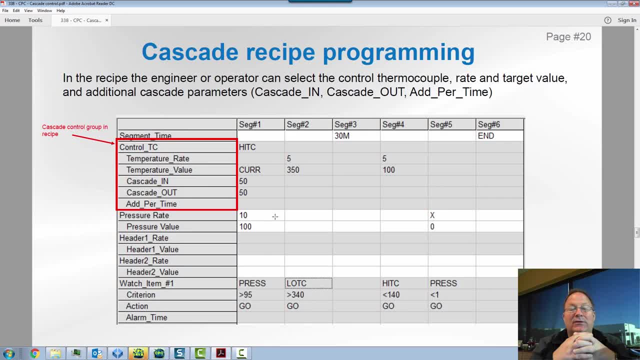 Okay, And what would that look like when you actually bring up the recipe? Well, it looks like this: It basically gives the operator a selection of a control TC Allows him, Allows him to To provide rate and value and cascade in, out and add per time program that in the recipe. 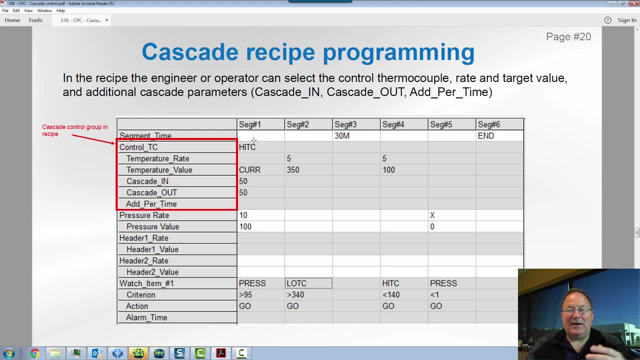 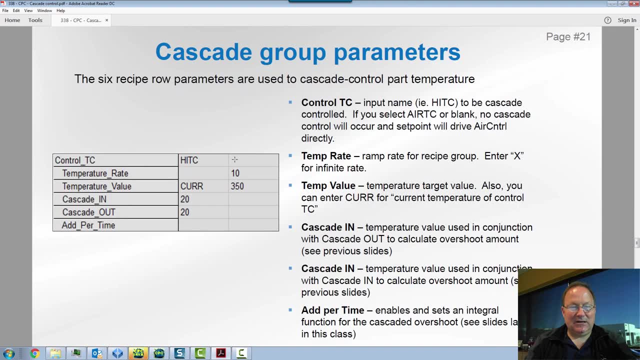 and this is a small example. we'll be going into more later on. So that is the setup for the recipe. And what are these? what are these parameters do? well, the control TC is basically the name of the input you want to control by, and again, you can control by an individual part: thermocouple. 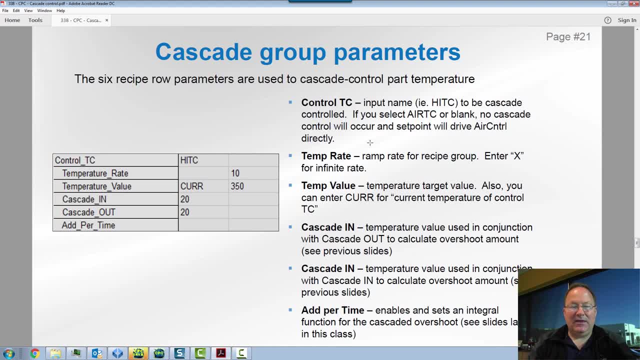 or you can use high TC, low TC, average TC. if you select air TC, we've already told the output object to to disable cascades for that. so by by adding air TC here you're- you're actually telling it the system to to turn off cascades, okay, or to turn off cascade control. 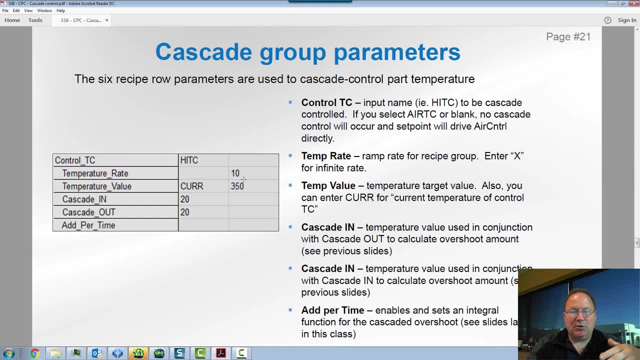 temperature rate will be entered in degrees, degrees per minute. you can put an X there for an infinite rate. if you want it, just to rock it up to the, to the, to the value, temperature value, It would be the that that the target of the of the rate, or you, if the rate is X, out it's. 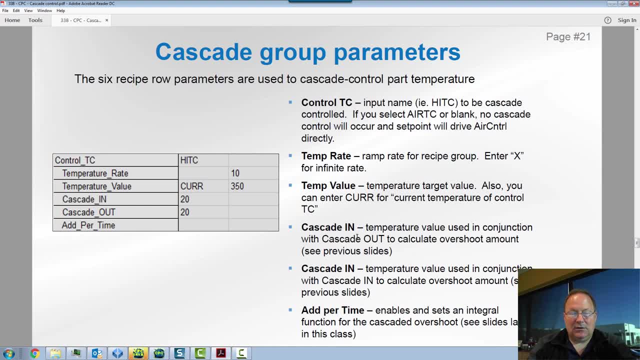 basically what temperature you want to control by toward control to, and then cascade in and cascade out. actually, this is an error. that should say cascade out. Those two values are obviously creating that ratio and the cascade out is also creating the, the limiter that we talked about before. 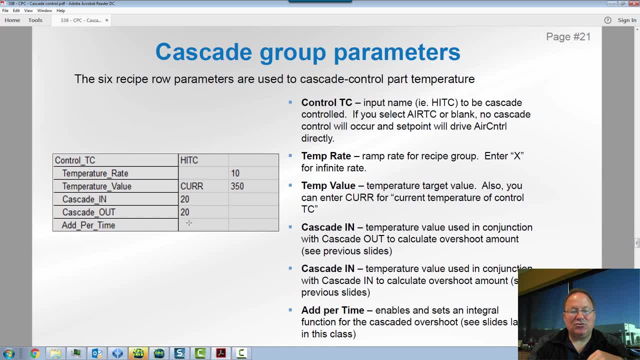 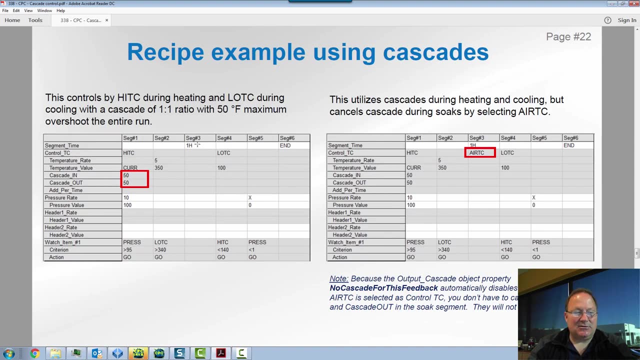 Add per time is another function that we're going to talk about later in this, in this training. It's an integral sort of a, a change to the overshoot based on a certain deviation over time. okay, so that that's a definition of those properties, and here are some examples. so here's. 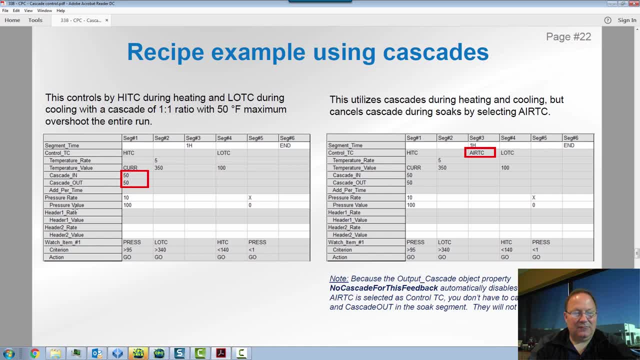 a case where I'm using a one to one ratio of 50, 50, 50, cascading the casket out. this, this tells me. I'm going to limit my maximum overshoot to 50 degrees as well, and I'm going to leave that during the entire run. the only thing I'm going to, I'm going to change is 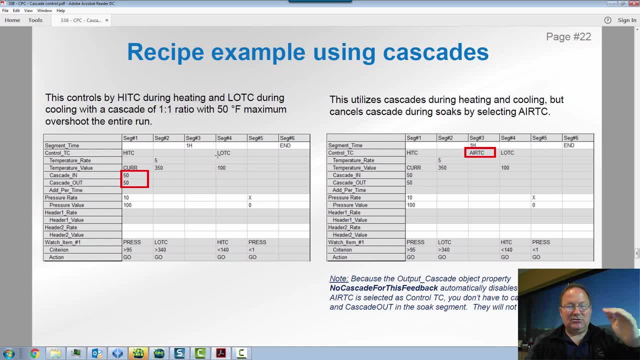 I'm going to go from high TC during the during the heating and the Soak, to low TC during the during the you know cooling. so I'm not going to switch my, my control thermocouple for my cascades and that would be a typical, very conservative type of up. 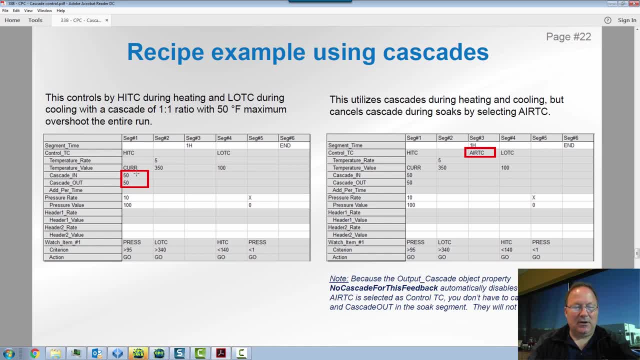 run where we- this would be considered a, a conservative, you know- cascade setting. as I said before, there are cases where, during soak, you, you might, you know, once you're, once you've driven your, your part up to step, going up to temperature, Yeah, need cascades during the actual soak period. and so sometimes what we'll say is either 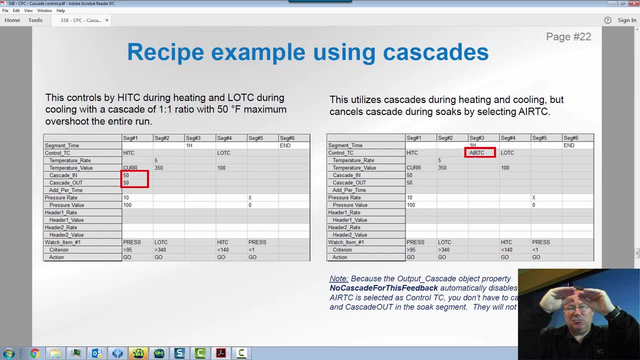 reduce your in to out ratios, to be much more conservative during that part, because what we don't want is a little bit of back and forth oscillations that might occur during cascading, or we can just basically switch to air TC control and that will eliminate all cascades during that soak period, and so you're going to see this often on and you 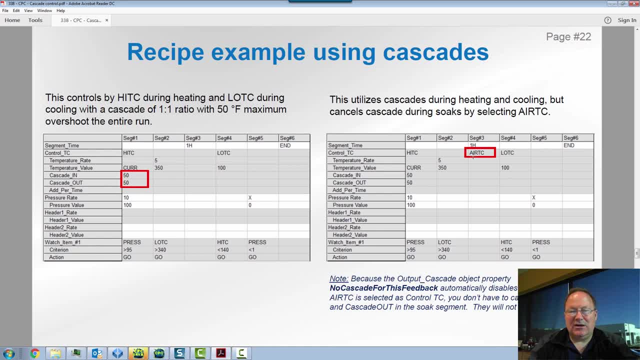 can counsel customers to use air TC in soak periods to give them a nice straight line. You can also leave high TC in there as well, but it's advisable not to have a high out to in ratio during that time. And obviously, air TC being put here, that no cascade for this feedback. property of the. 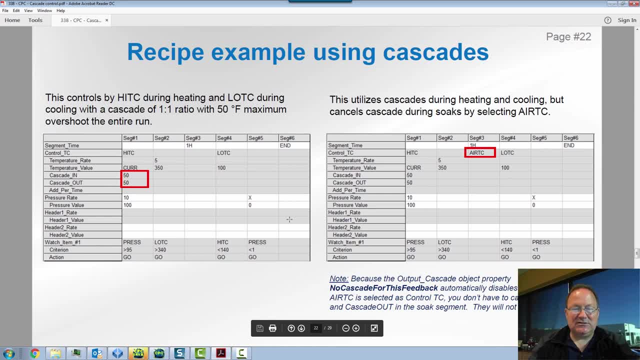 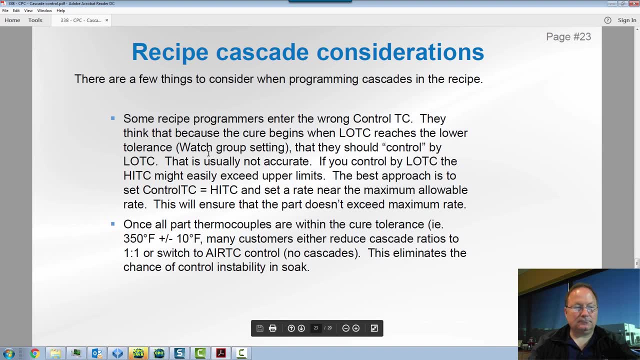 output object will eliminate cascades, and then we switch back to low TC during cooling. So what are the considerations here? There are a few things to consider when programming, So remember that one of the things that you'll see is that operators and engineers tend to 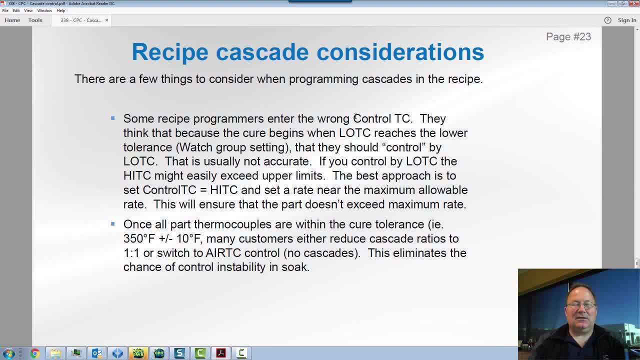 want to put the wrong control TC in. They think that because the cure doesn't start until the low TC hits the lower threshold, they want to control by low TC. but that's an incorrect assumption. You want to push them to try. You want to control by high TC, which would be the highest temperature and the quickest. 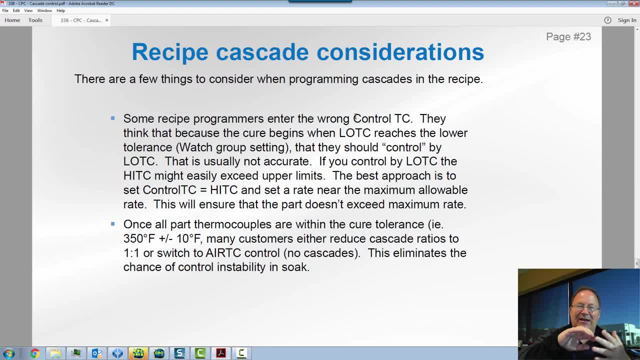 heating thermocouple and try to push that at near the upper band of the maximum rate. So if the rate is 5 degrees a minute maximum, you might want to control high TC to 4 degrees a minute and then drive it to the upper band, upper tolerance or near the upper tolerance. 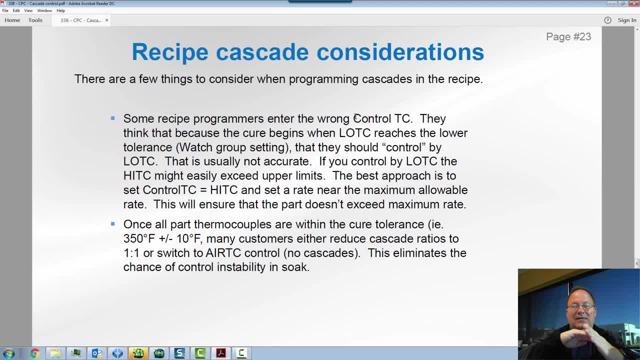 and that's going to give you your best control while still maintaining the maximum limits, because if you control by low TC, You might have a situation where it's driving trying to drive low TC up, but the high TC goes over rate, it goes over temperature, and so that's usually not something that they want. 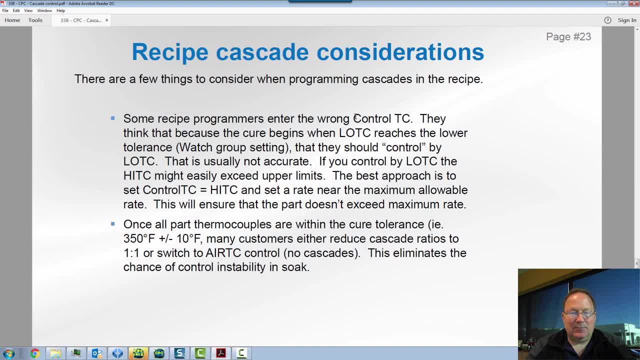 to see and it will create part rejections and that type of thing. And the other consideration is: when you get into soak, remember not to have a high out to in ratio and or switch to air TC control at that point. So that's a. 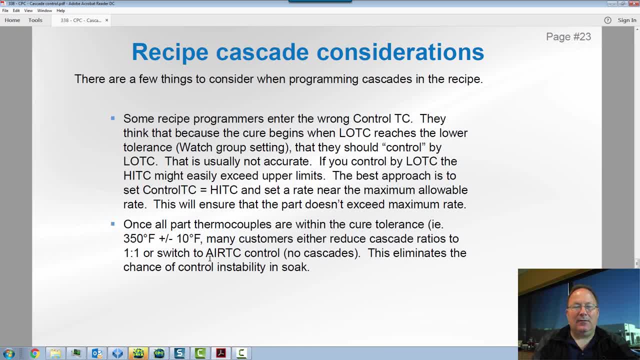 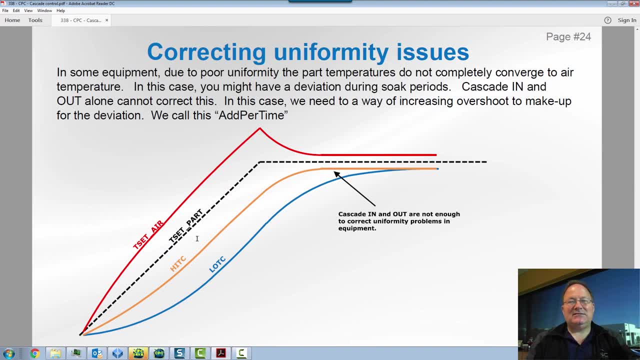 Those are just good recommendations to avoid instability during a recipe. So there are cases now where ovens or autoclaves might be a little bit non-uniform in their temperatures. So let's say you're running in a piece of equipment and when you get up to soak air 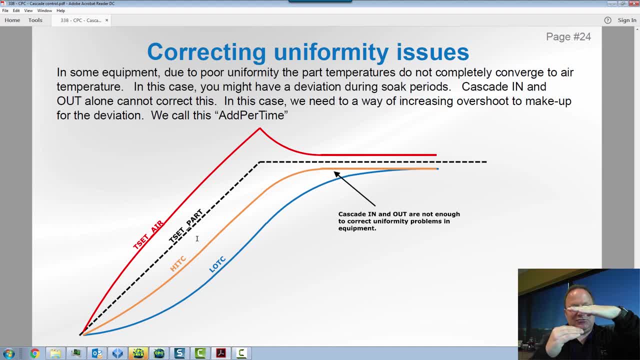 temperature goes to 350, but the part temperature is always hovering below that. Well, if you're using cascades, cascading and cascade out is a proportion of the deviation. So if I use a one to one ratio and my part temperature is sitting three or four degrees, 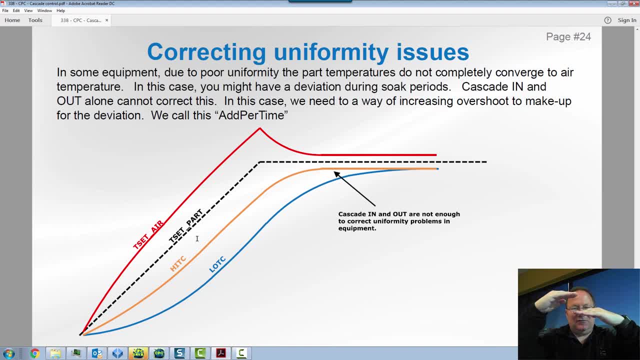 away from set point during soak, my air temperature will be three to four above and it'll just stay there forever. And so you would end up with this. Even though the part is with intolerance, it never actually gets up to final set point, because those cascades doesn't. 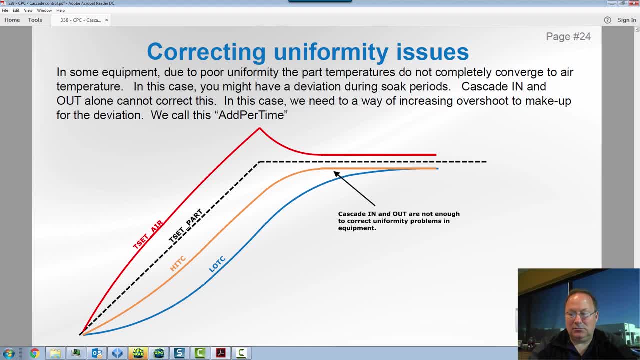 It will. It will not handle that. that the uniformity problem. Okay. So in this case, what we want to do is provide an extra boost to the overshoot based on this deviation, this sort of extended deviation, And for that what we will use is is at per time. 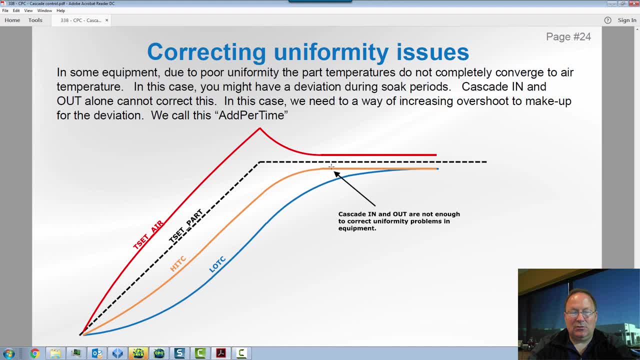 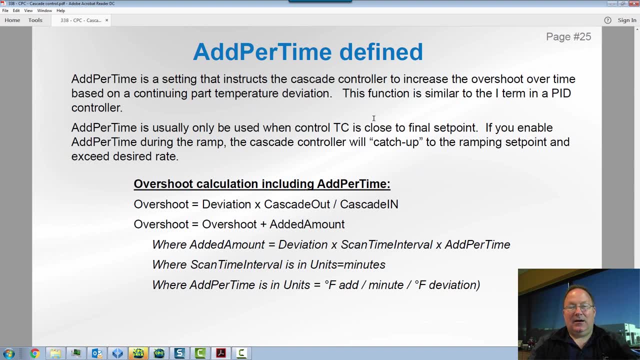 And that's a. that's a function used to to eliminate that deviation or that error at soak. And what is it after? time is defined as a? basically, It instructs the cascade controller to increase the overshoot over time based on a continuing deviation of the part temperature. 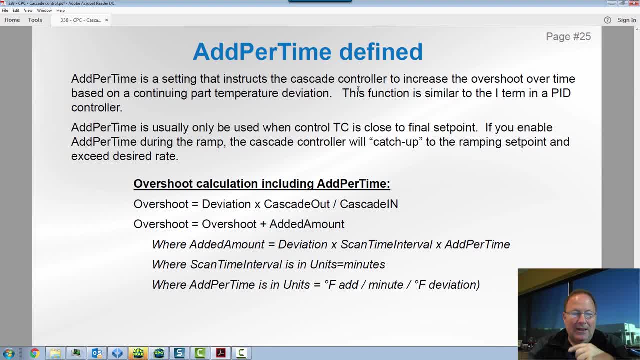 So it's very, very similar to the I term in the PID controller And we usually want to use that when we get close to final set point, because we don't want to use it during ramping, because what it's going to do is drive that, that control. 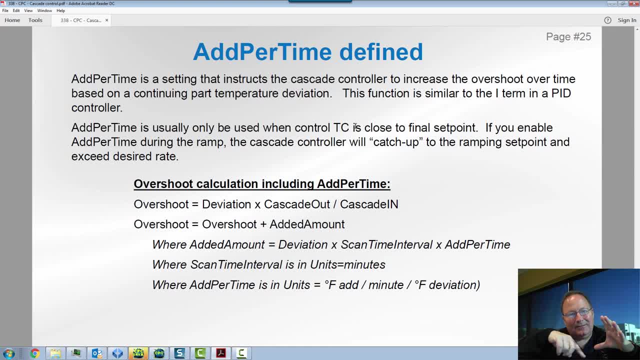 thermocouple back up to set point and we're going to end up with that catch, the catch up problem where we're exceeding rate. So here's, Here's how it, how, how the calculation works. so the overshoot, as we talked about earlier, was deviation times: cascade out over, cascade in, and then we're going to add to that overshoot. 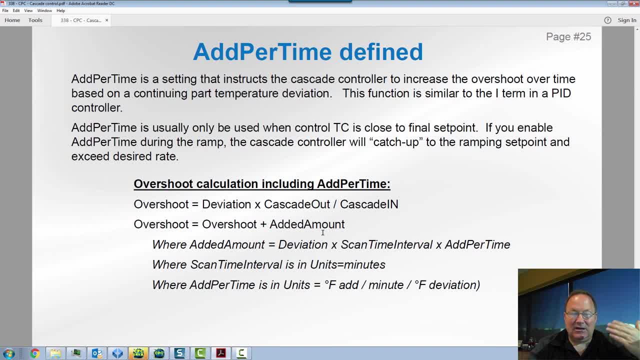 a special amount is going to be added every cycle, every scan time, and basically the added amount is equal to that deviation of times, the actual time in minutes Times, And then we're going to add per time. you know constants. so the the upper time constant is: 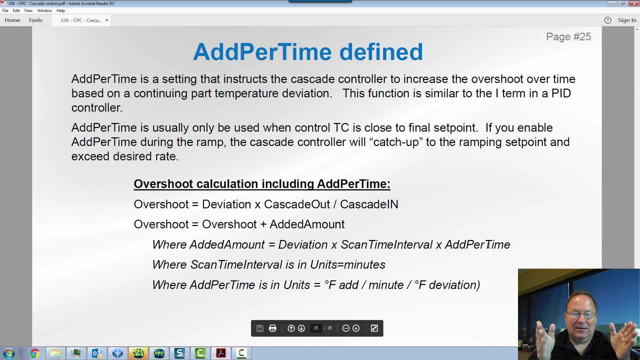 the is a gain or a multiplier on the on the at that deviation times time. so So scan time interval is usually in minutes, so but but it's going to be calculated every task or scan interval and then at per time is in units of degrees F added per degree. 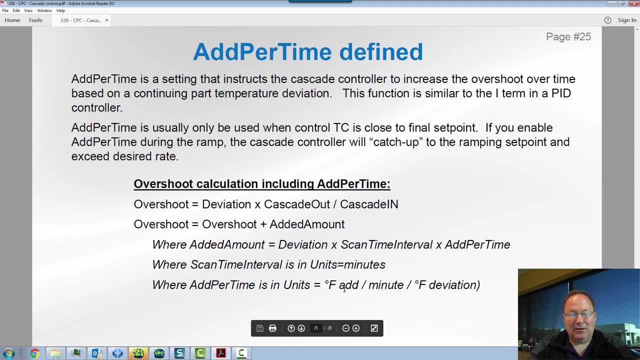 minute per minute per degree F deviation, and so basically, if I'm deviating one degree for one minute, If I and I have a at per time of one, then it will add one degree to air temperature per minute, right? so that's basically a lot like the integral function of the PID. 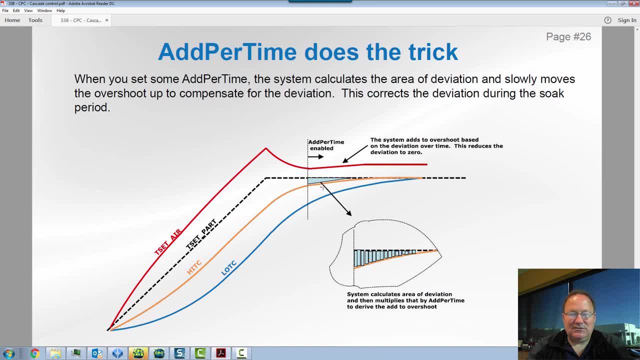 And what that does for us, is it? it's, it basically solves uniformity problems. because here, here you, you can see, you know, if I initiate at per time, as my control thermocouple comes close to set point, it begins to integrate or calculate the area between, between the 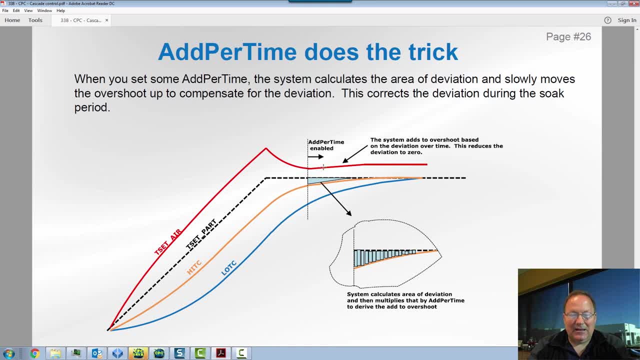 of of that deviation, basically, and we're, and we begin adding to the overshoot and so we allow that high TC to drive up, and this then becomes sort of handling uniformity problems and we end up with right on top of set point and the air temperature then will maintain. 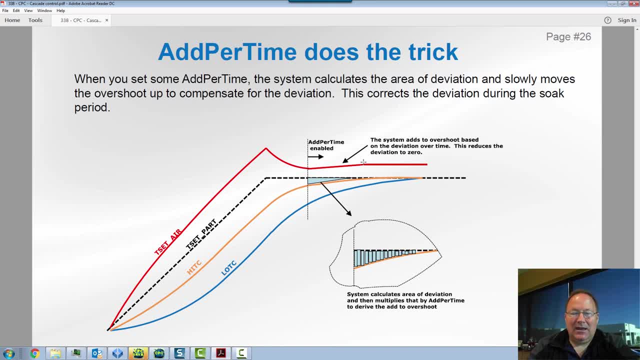 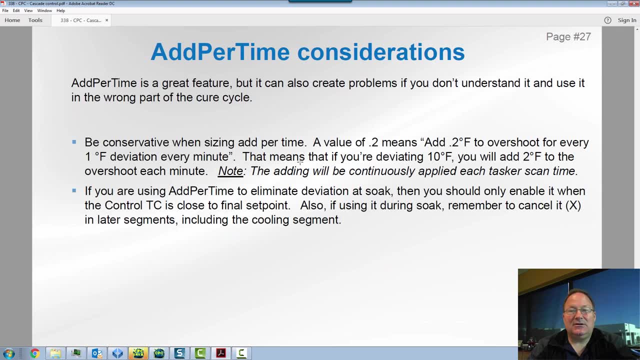 this sort of elevated overshoot and and so that's that's how at per time works and it it works very, very well, but there are some, some considerations. you know a lot of people who Who use it will use it incorrectly or they'll put too much at per time and create instability. 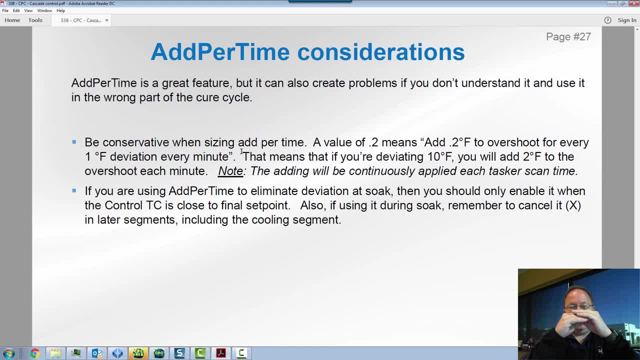 so be conservative. when you're sizing it, remember that it's looking at the area under the curve. so if I'm deviating by ten degrees and I have a a high at at per time, I might end up with with a very quickly rising overshoot. so so if if you use a value of point to what that, 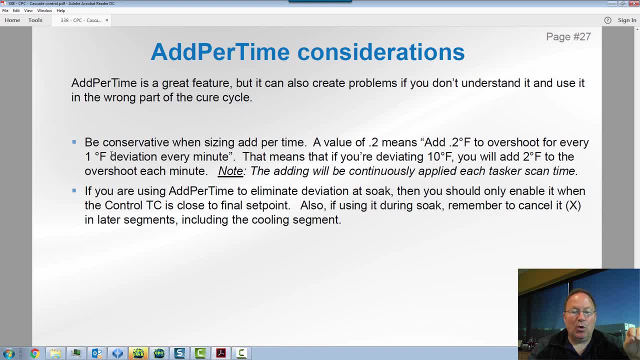 means is that you're going to add point two degrees after To the overshoot for every one deviate, one degree of deviation per minute. that means that if you're deviating ten degrees you will add two degrees per minute to the overshoot and that is that as a deviation decreases than the overshoot amount will also, or the 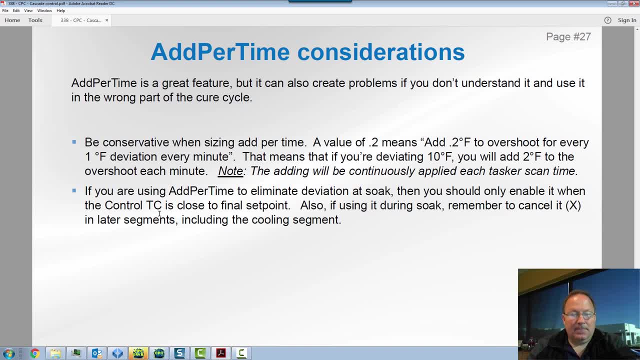 the add to the overshoot will decrease. If you're using it for time to eliminate that uniformity problem during soak, then make sure that you only turn it on when the controlling thermocouple comes close to set point, and I'll show For example of that. and then, once you're done with the soak, you you want to exit out, or 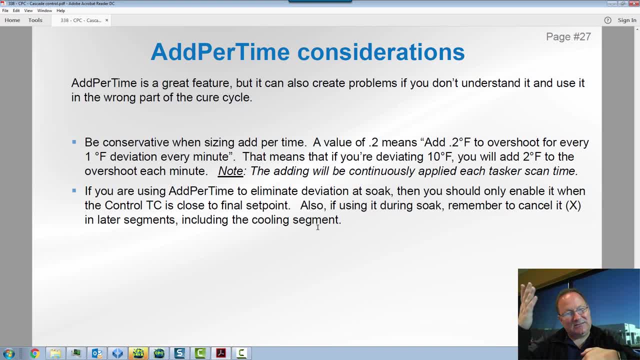 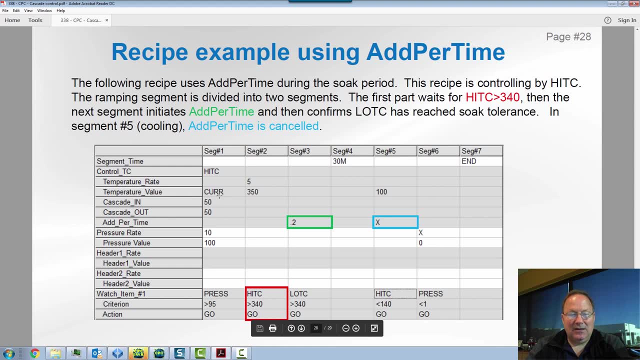 cancel that at per time. you don't want it to function during cooling because it'll play catch up again. So here's an example of using at per time in a in an actual recipe. so here we are, controlling high TC at five degrees in up to three fifty, but normally we would wait until low TC gets. 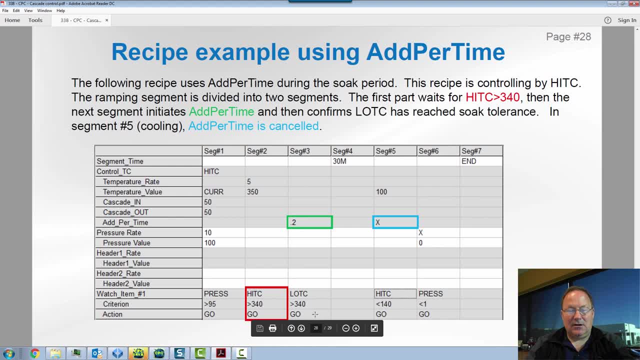 greater than three forty. but we've added a second, a second segment here, and we're saying three forty, which is within ten degrees of set point, then we move on, and the only thing I'm doing in this segment is adding is creating an ad for time of point two. so that's where